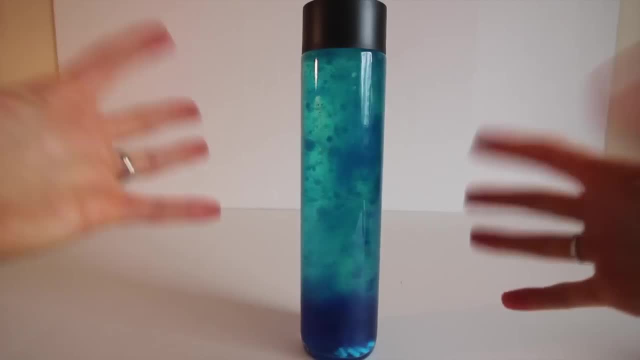 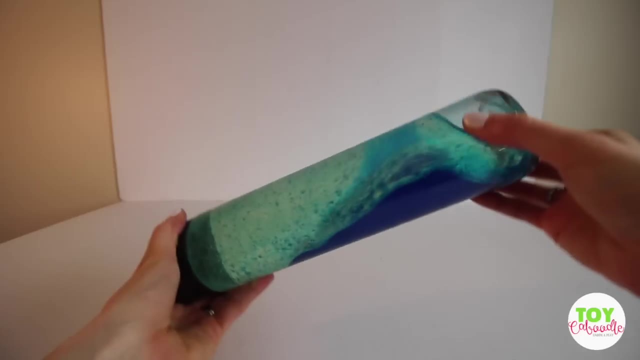 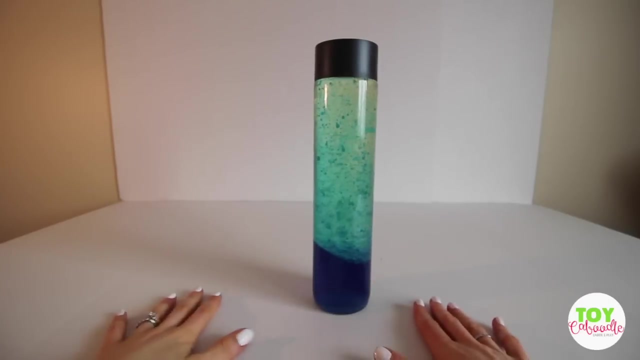 Alright, you guys. I closed the top because it was going to start spilling over Toy Kaboodle. Hey guys, welcome back to Toy Kaboodle. Today I'm going to be doing a do-it-yourself lava lamp. How cool is this? I'm going to be showing you guys how to make this with just simple everyday household items that you might have. 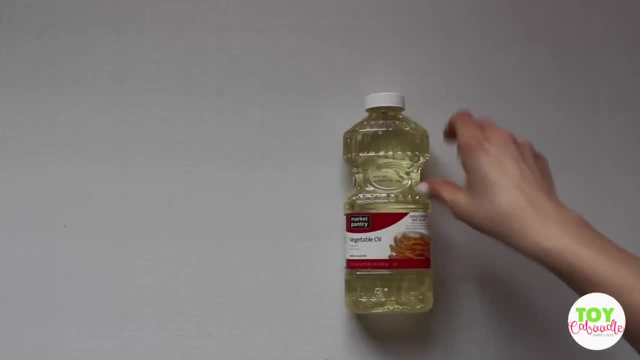 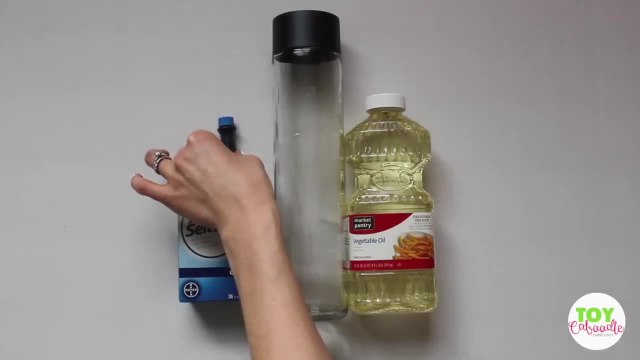 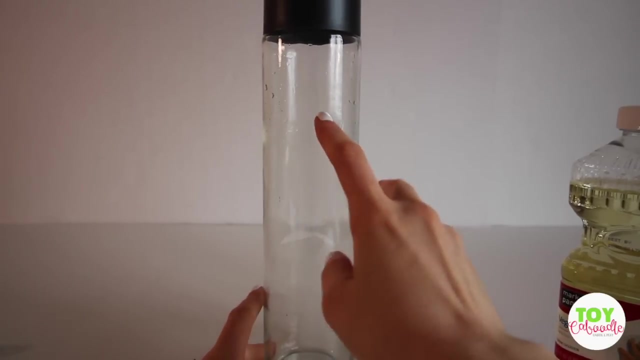 So what you're going to need is you're going to need vegetable oil, you're going to need a glass container, you're going to need some Alka-Seltzer tablets and you're going to need some food coloring, And so what you want to do is you want to fill up your glass container that you have with vegetable oil up until right about there. 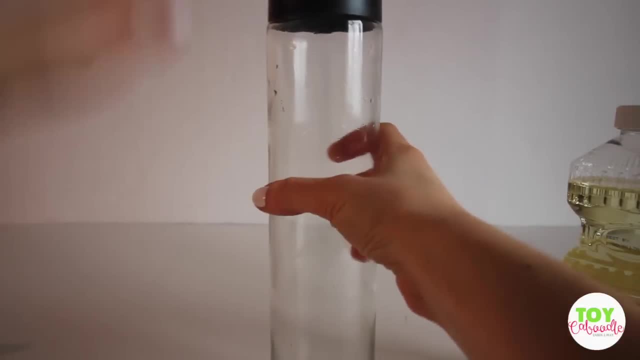 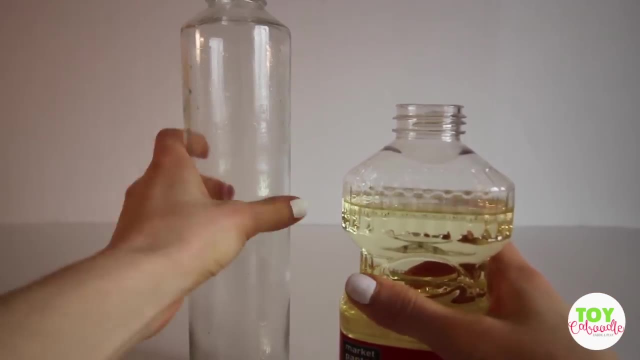 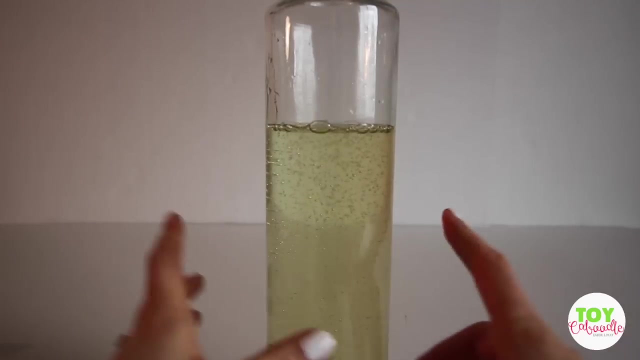 Three-fourths of the way with vegetable oil. So let's go ahead and do that. I hope I have enough, You guys. next we're going to fill this up with water. Alright, you guys. so I do have some water here. It is room temperature. 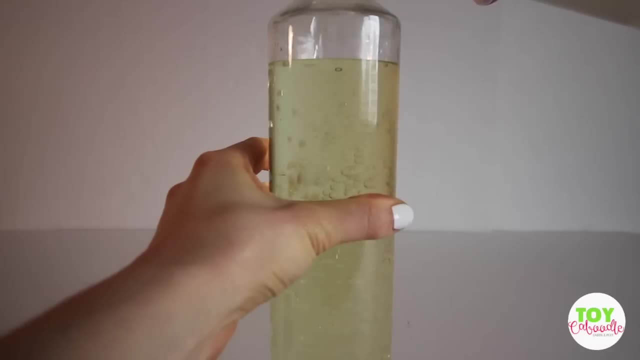 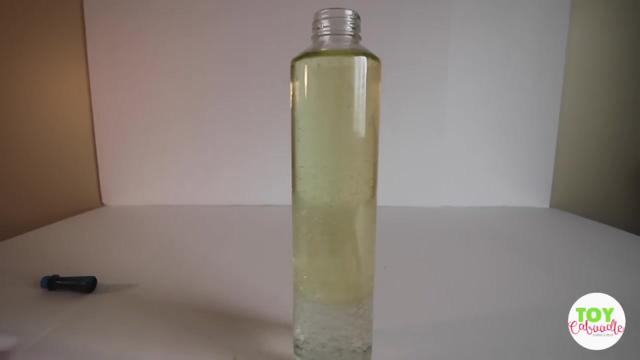 And we are going to fill this up until about an inch away from the top And, as you can see, there I left a little bit of spacing. Alright, you guys, I had to zoom my lens out a little bit because I want you guys to see what I'm doing. 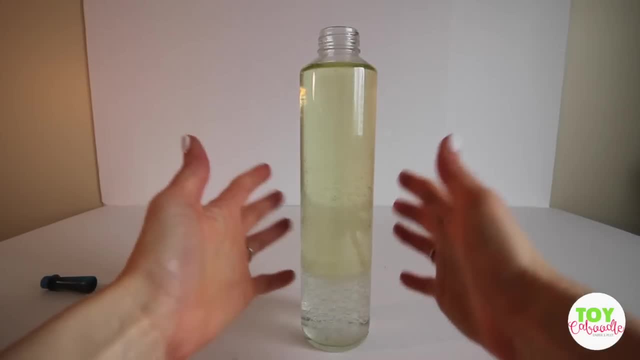 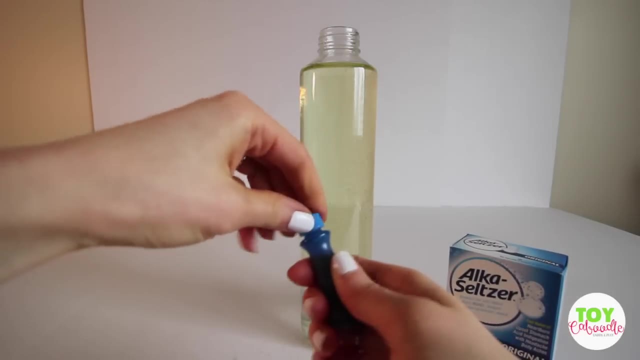 I want you guys to see the whole reaction, how this actually happens. So then I have my Alka-Seltzer tablets and I have my food coloring. So what I'm going to do is I'm going to add about five drops of food coloring. 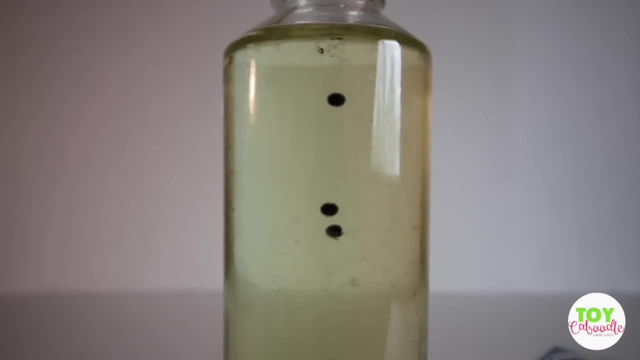 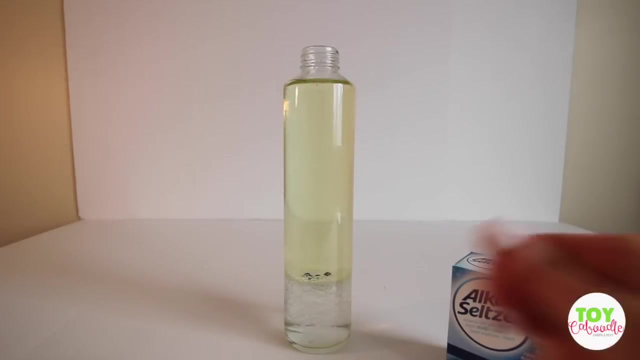 Or maybe I'll add a little more Just like that. Alright, you guys, let me screw on my food coloring before I get that everywhere. Alright? next you have your Alka-Seltzer And then you have your Alka-Seltzer tablets. 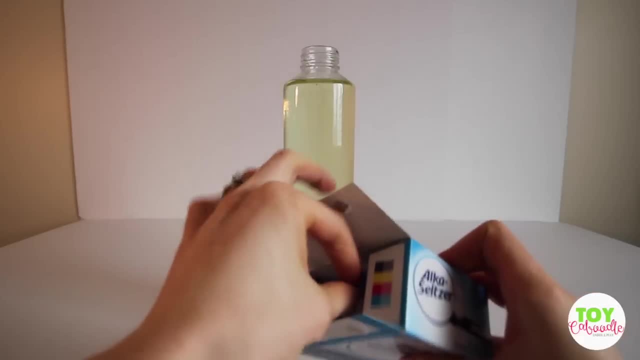 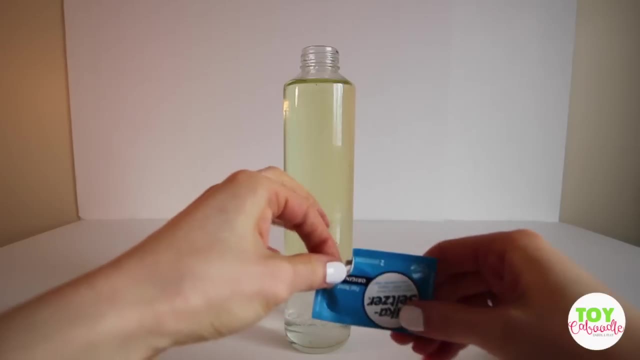 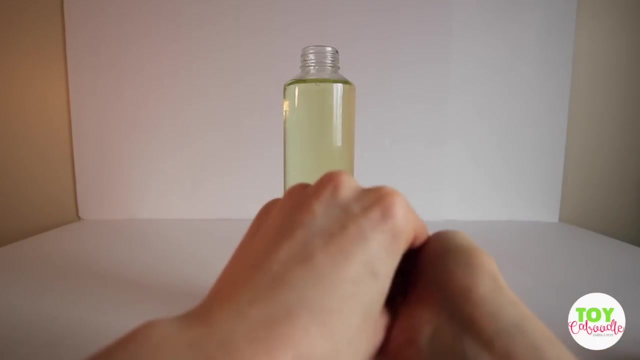 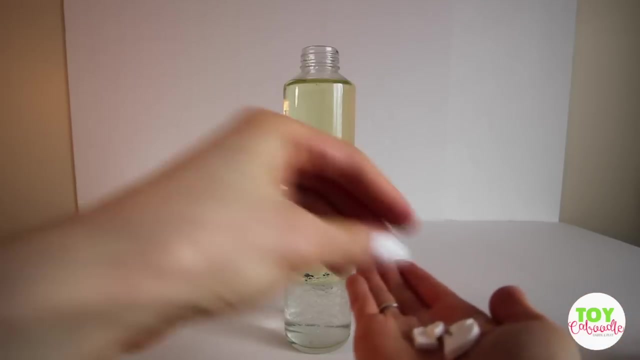 And really you just need one tablet, but you have to break it up into pieces, So looks like there's two in a package. We're just going to take one out And I'm going to break it up into some pieces, Just like that.